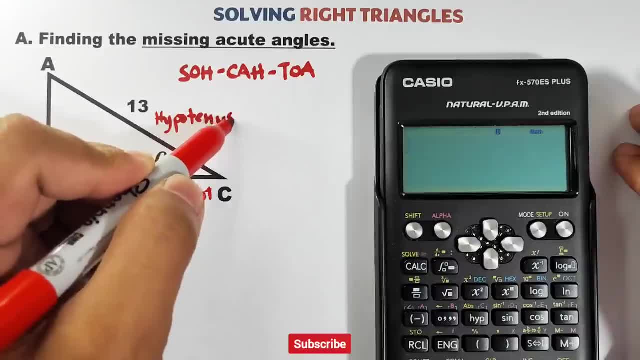 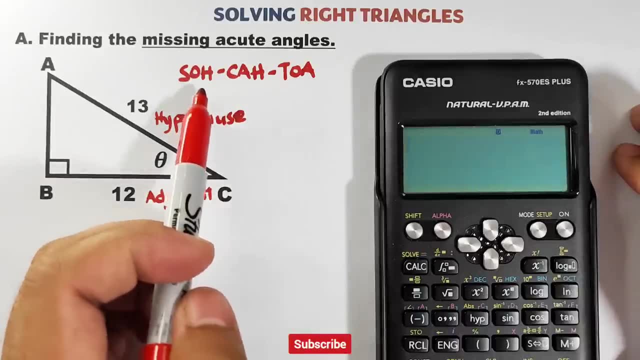 hypotenuse. Now, since you have your hypotenuse and adjacent side alin sa tatlong to So SO KA and TOA ang merong adjacent and hypotenuse. Yes, you're correct, Definitely the KA. 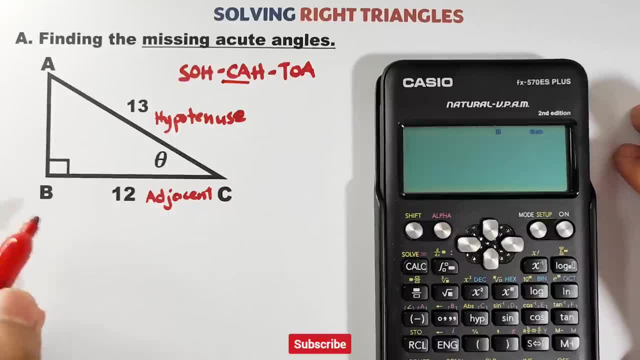 Meaning we will use our cosine ratio. We have here cosine theta is equal to adjacent over the hypotenuse Substitute. the value of adjacent and hypotenuse We have cosine theta is equal to 12 over 13.. And to use this calculator, 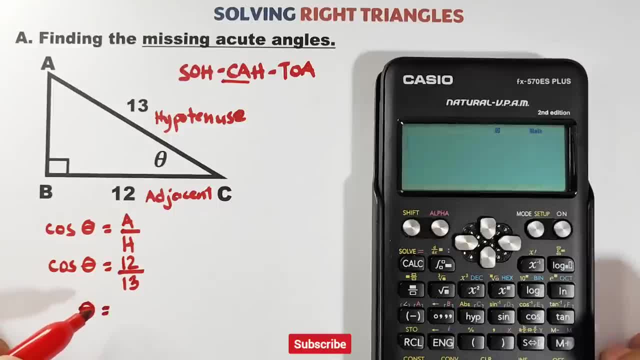 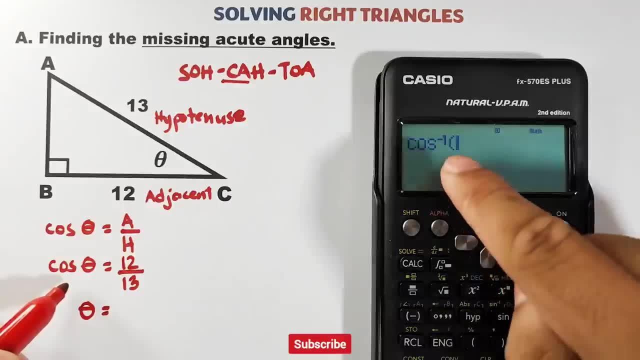 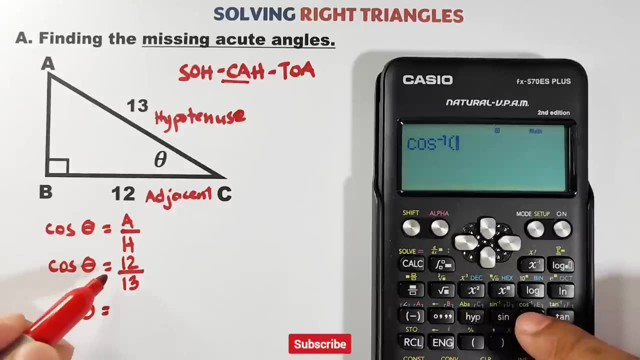 get the angle, theta, All we need to do is to press shift and then press cosine, Dapat ang lalabas dito, guys, ay yung may negative 1. Again shift, then cosine, Then after that input your 12 over. 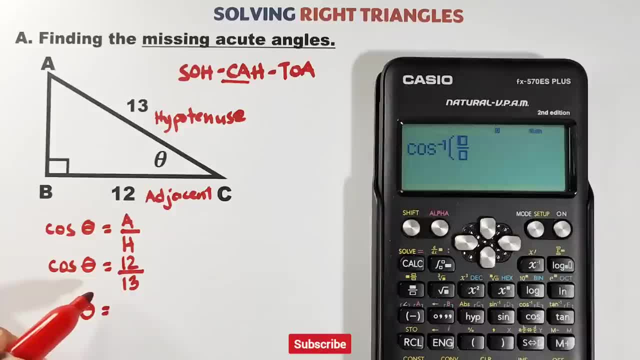 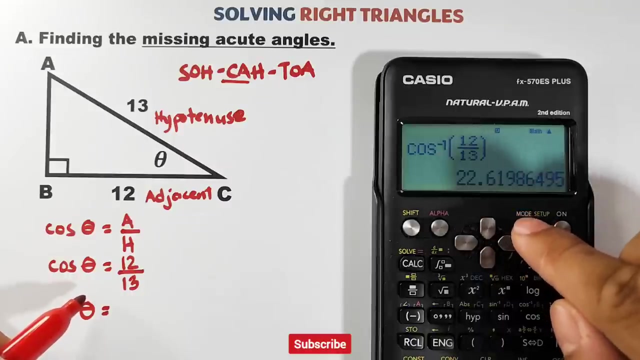 13.. That is this one the fractional symbol. Input your 12 in the numerator and 13 in the denominator. Close parenthesis After inputting after shift cosine. then the fraction 12 over 13,. you can press the cosine. As you can see, ang lumabas dito is 21.61986495.. Ang kailangan natin is ang angle. So in your 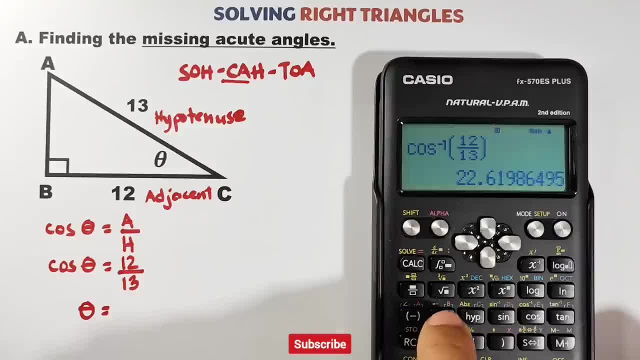 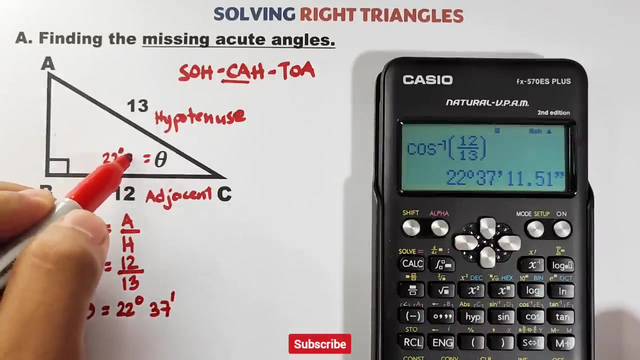 calculator. you can press this DMS or degree, minute, second, itong symbol na to Press mo to At itong lalabas. As you can see, meron tayong 22 degrees, 37 minutes and 11.51 seconds. Hanggang dito lang tayo sa minutes. Okay, So our theta is 22 degrees and 37 minutes. Ito yung value niya. Now lagyan natin dito. This is 22 degrees and 37 seconds. 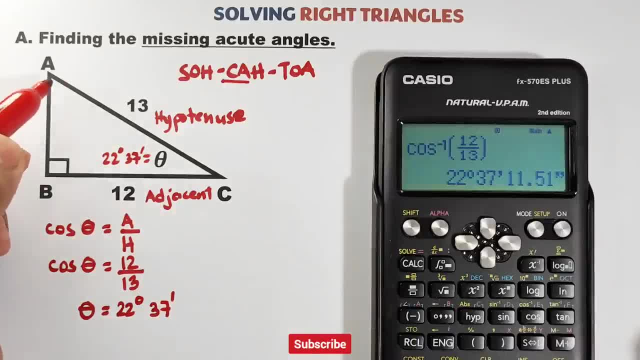 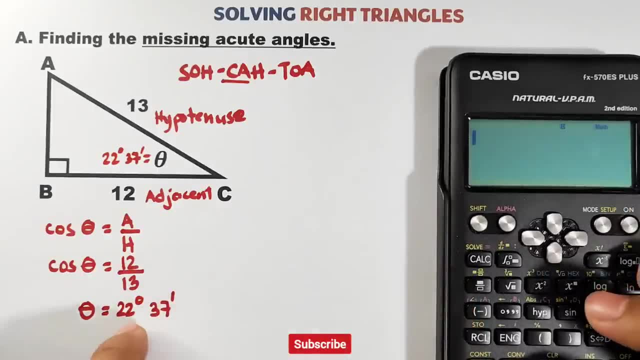 Now, if your teacher asks you about the measurement of this angle A, pwede naman natin siya makalculate. So ang gagawin natin ngayon is that we will subtract this from a 90 degree, Kasi, alam naman natin the three angles is equal to 180, meaning this two will share on the sum of 90 degrees. So we have 90 degrees minus your 22 degrees. 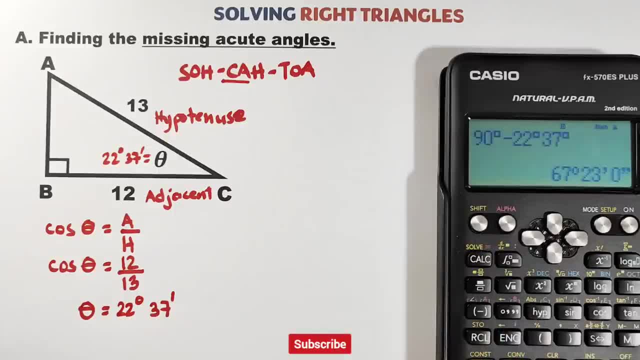 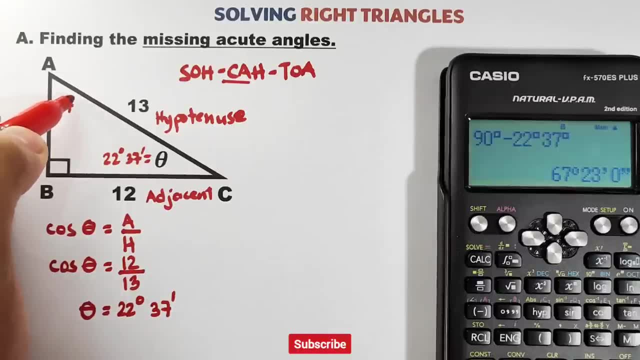 and 37 seconds, And the answer is this: This angle is equal to 67 degrees and 23 minutes. I hope, guys, na nakuha niyo na yung first example natin. Now let's continue with the second example. I hope, guys na nakuha niyo na yung first example natin. Now let's continue with the second example. 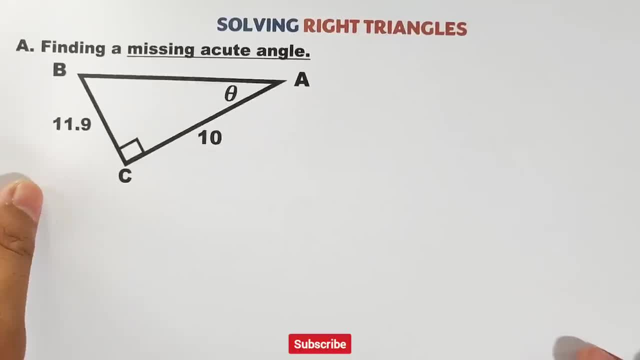 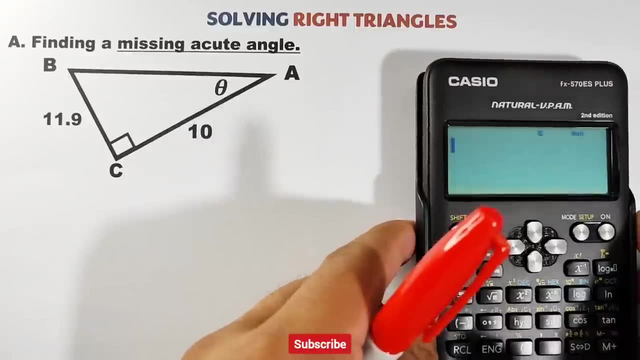 First is look at this sign in forzesinda, yung preparasyon ng modem Nagagawa niyo bumabi sa palyagan. For our second example, this is the right triangle and we will still use this calculator. Now let's put our SOH CAH TOA. 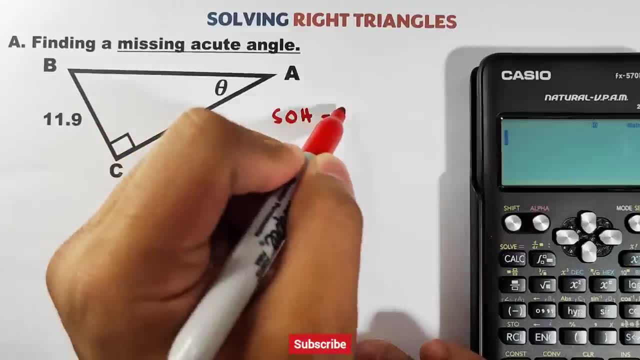 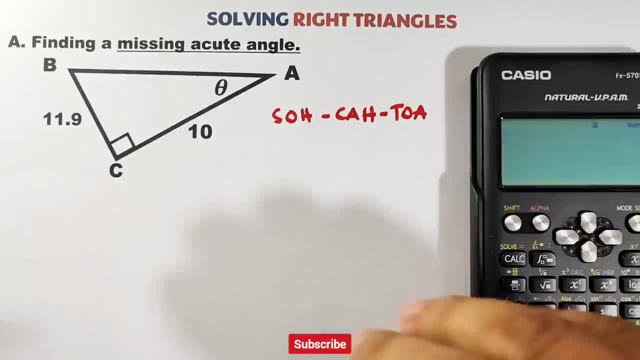 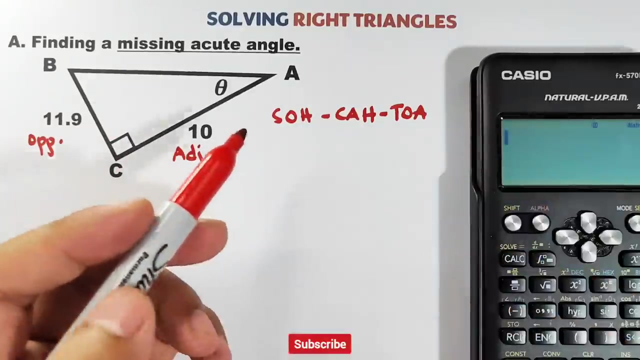 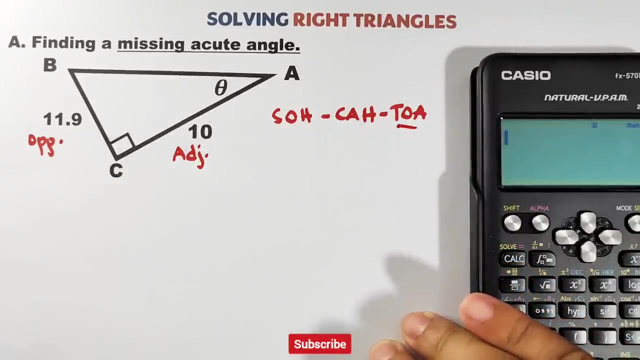 SOH CAH, TOA. With respect to your angle theta, this side is the opposite Opposite side And this side is what The adjacent side. So which of these three has opposite and adjacent? Okay, very good, That is the TOA, meaning we will use tangent. 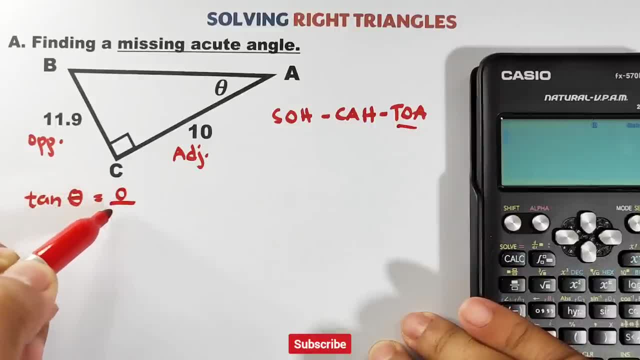 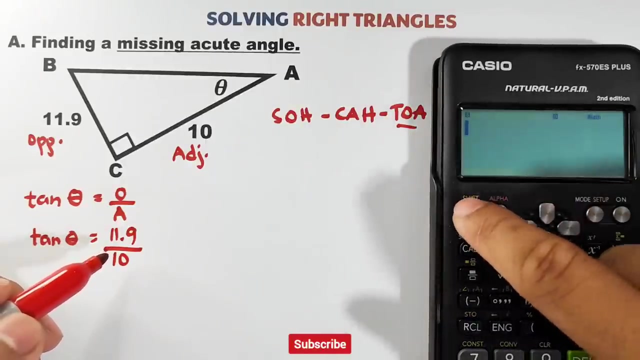 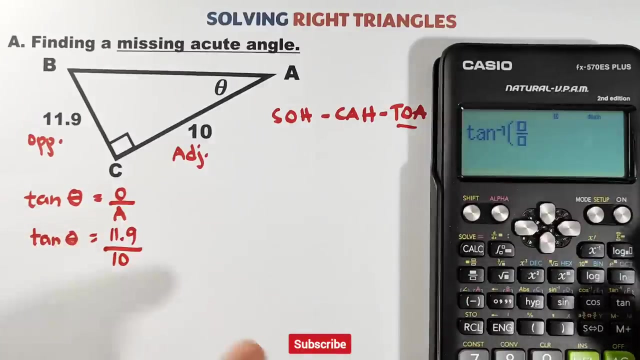 Tangent theta is equal to opposite over the adjacent side. Let's substitute the value Tangent theta is equal to opposite, which is 11.9, over your adjacent, which is equal to 10.. Same process, guys. We have to press shift and then tangent in fractional symbol and then start with 11.9 over 10.. 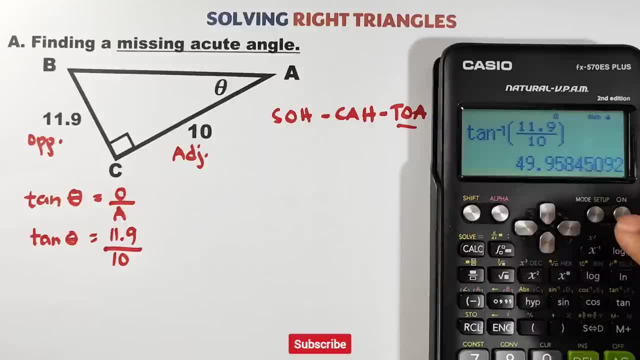 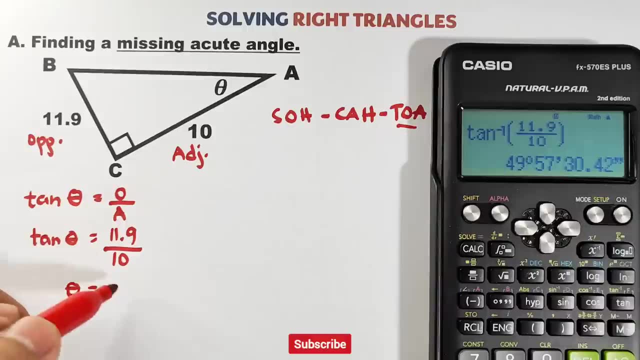 Press equal sign. This will come out, But we only need the angle Your theta is equal to for this DMS, 49 degree and 57 minutes. This is the answer for item number 2.. So, guys, if you want to find the angle B, just subtract it from 90.. 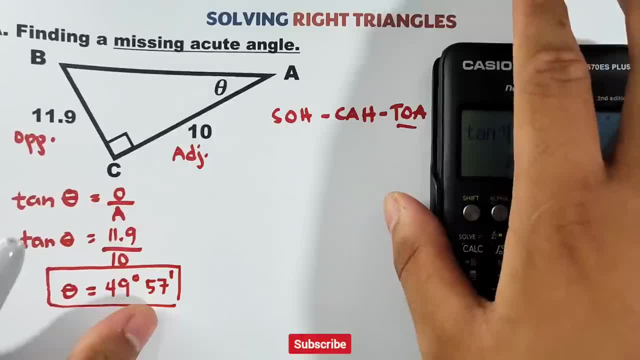 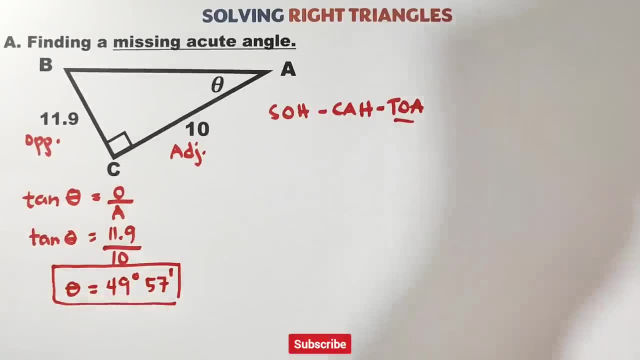 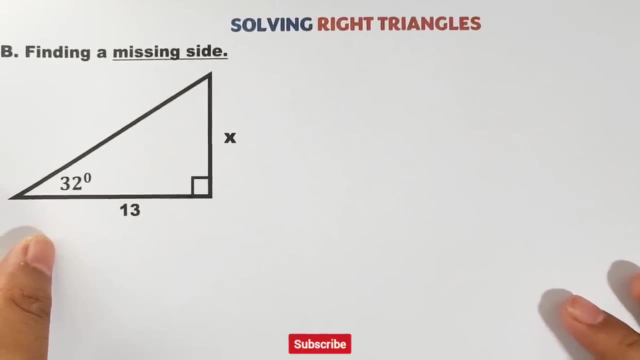 Okay, So that's it for the first part, And let's continue with the second part. In this part, we will solve for the missing side of a given right triangle. So how do we do this, sir? How are we going to find the missing side of a given right triangle if we only have one side and one right angle? 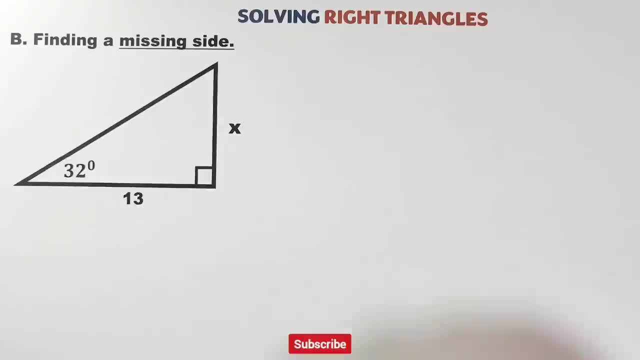 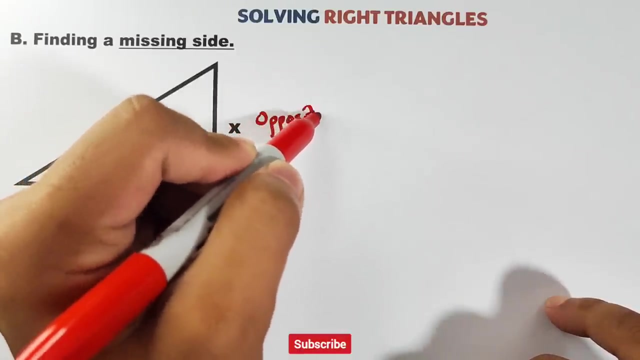 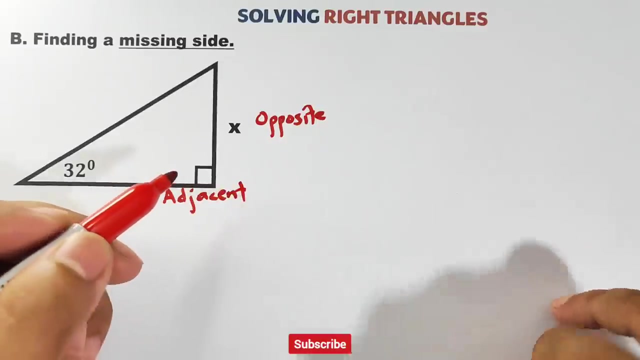 Don't worry because we can do it, So let's start. So here, with respect to this angle, 32 degrees, Our x is the opposite. What's missing is opposite, And this one is the adjacent. So again, it's the same again. 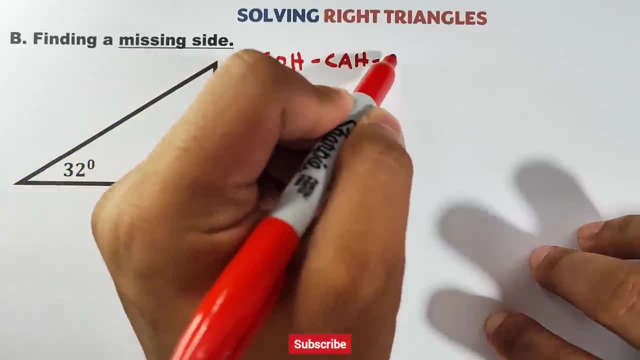 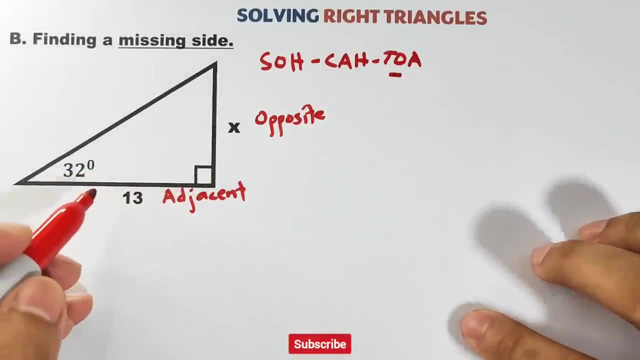 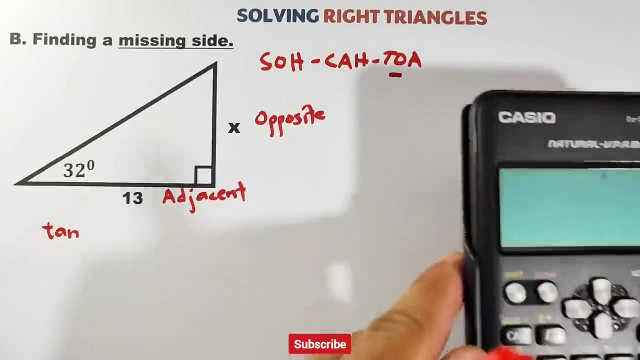 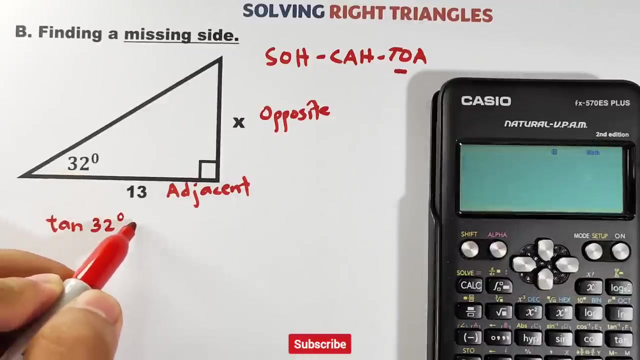 We have the opposite and adjacent, meaning we will use the same and our ratio is tangent. So, sir, how do we do this? We already have the value of our angle. Don't worry, because we can do it Tangent. 32 degrees is equal to opposite, which is x over the adjacent, which is equal to 13.. 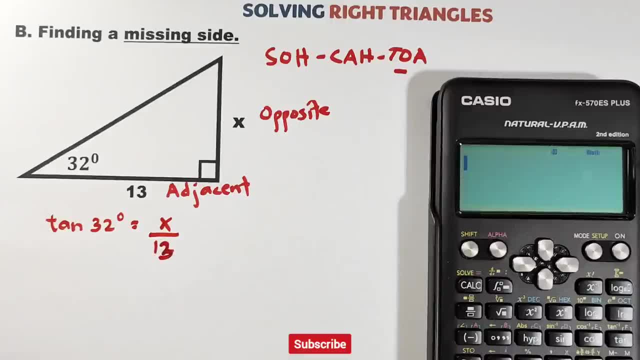 Now, as you can see what we need to solve for x, we need to isolate the variable x. Let's cross-multiply 1 times: x is x. This 13 times tangent 32 degrees, That is 13 tangent 32 degrees. 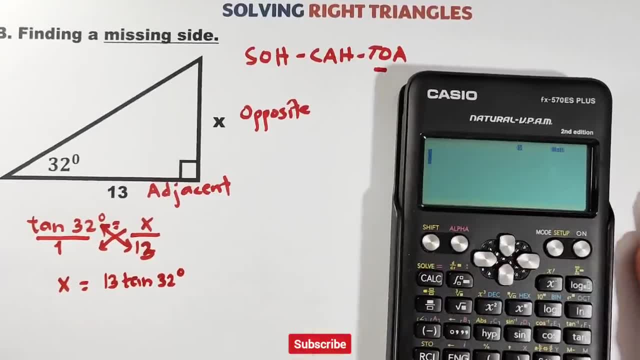 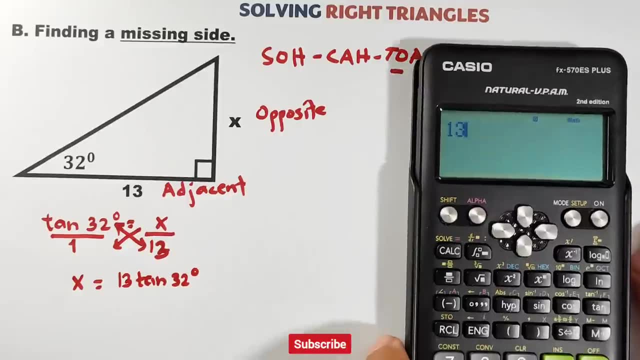 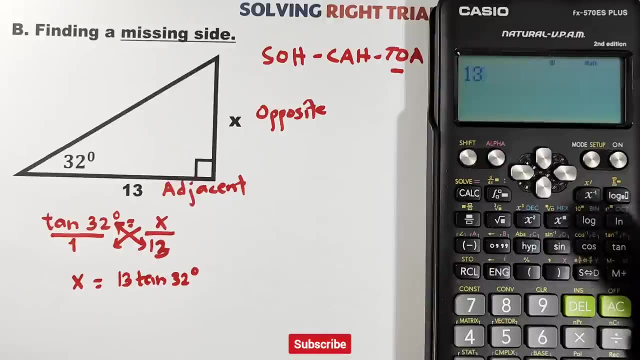 In this situation we only have input, But there is no shift that we can press. What we can do here is to input 13.. Okay, input 13.. Sorry, Let's do it again 13,, then tangent 32 degrees. 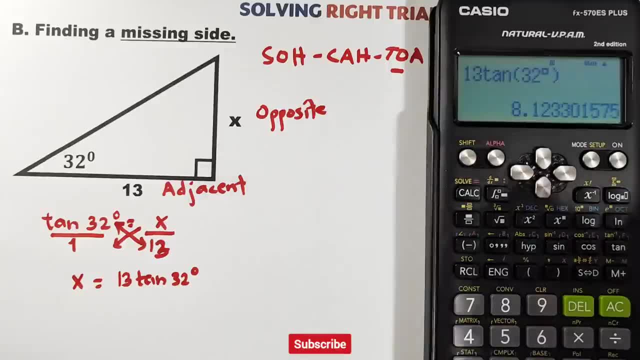 Close parenthesis. As you can see, this is what we have. No need to press the DMS or the symbol, because we don't need an angle. We are solving for the side. So our x is simply round off into two decimal places. 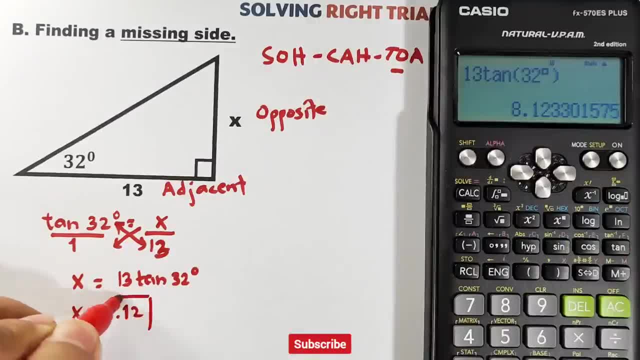 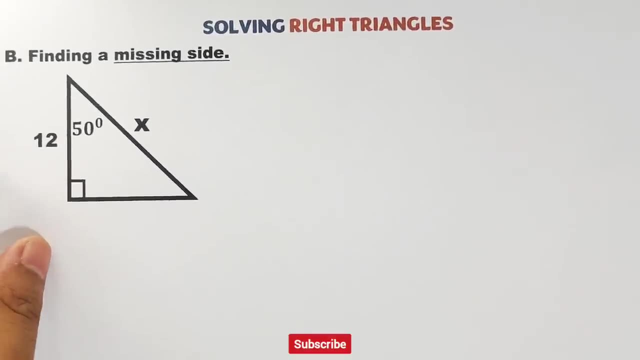 That is 8.12.. And this is the answer for item number 3.. Okay, guys, Now let's continue with the last problem. Here is our last problem. guys, For the last problem, find the missing side. Okay. 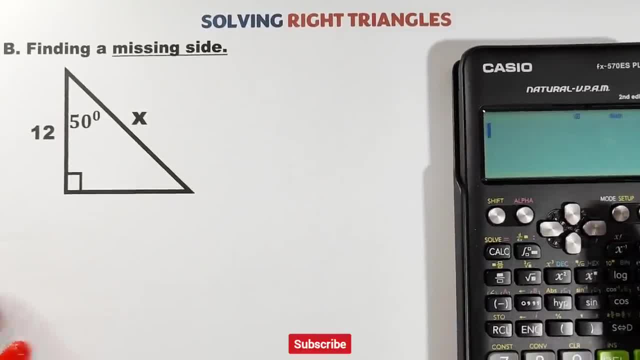 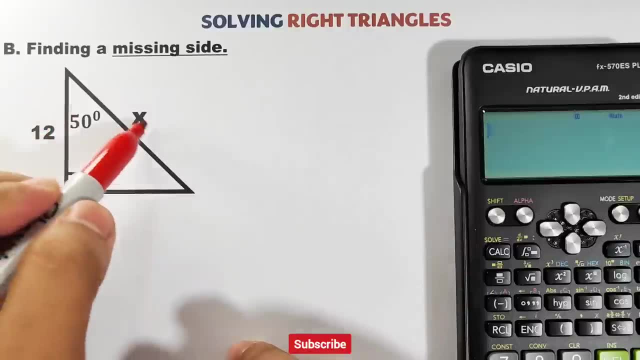 So how is this With respect to your 50 degree angle or acute angle? 50 degree, this is your hypotenuse And this one is your adjacent side. So what is adjacent to the hypotenuse in SOHCAHTOA? 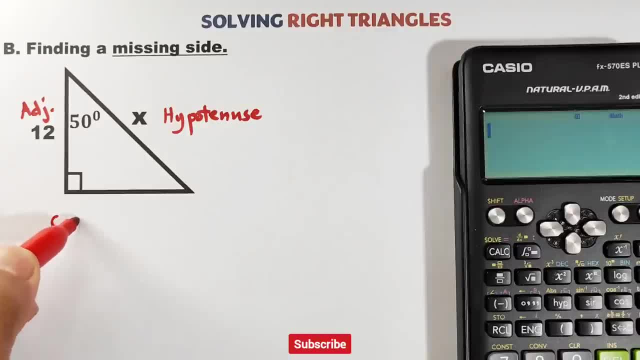 Very good, We will use the cosine, Cosine, Cosine, Cosine, Cosine, So we need to add another 50 degrees. argetine: Cosine, Cosine, Cosine, Cosine- 50 degrees. 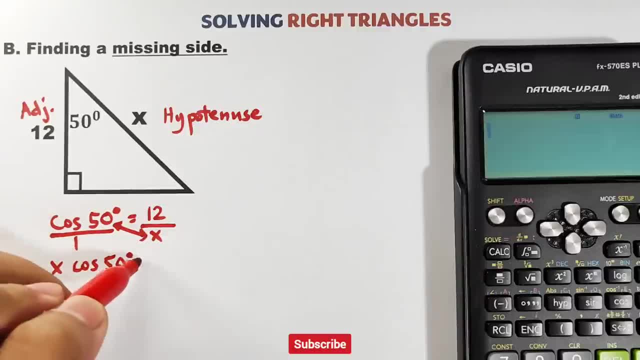 Casine 50 degrees. This is equal to adjacent, which is 12, over your hypotenuse, which is equal to x. Crossmultiply again This is x. divide both sides by cosine 50 degrees, and this one is also to be divided by. 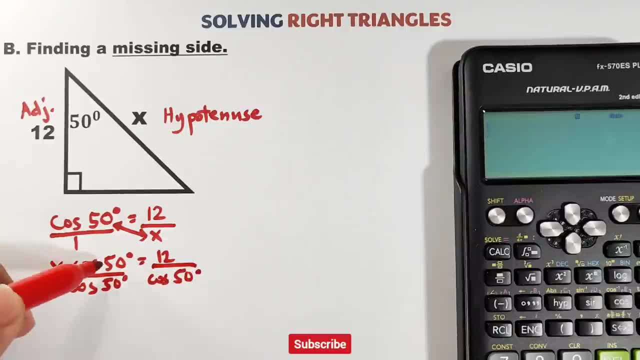 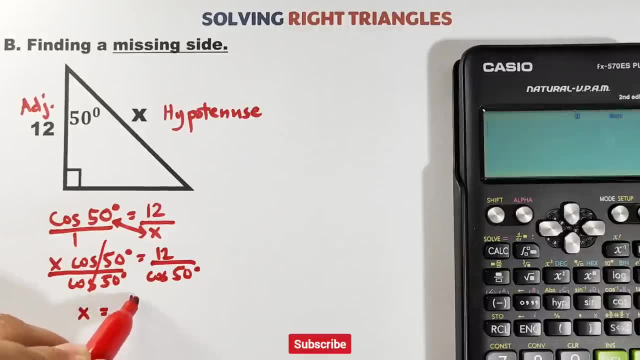 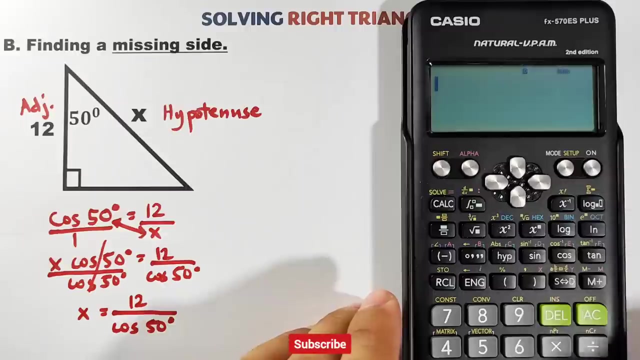 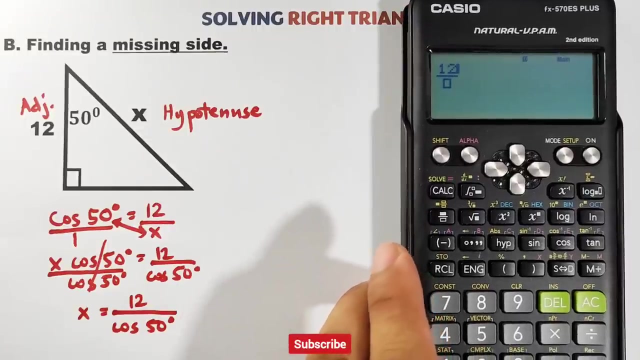 cosine 50 degrees. Let's cancel this. As you can see, we have an x-variable. x is equal to 12 over cosine 50 degrees. Now, sir, how is that? It's like this: Using your calculator, press the fraction, then 12 is the numerator, and then, for the denominator, press cosine.